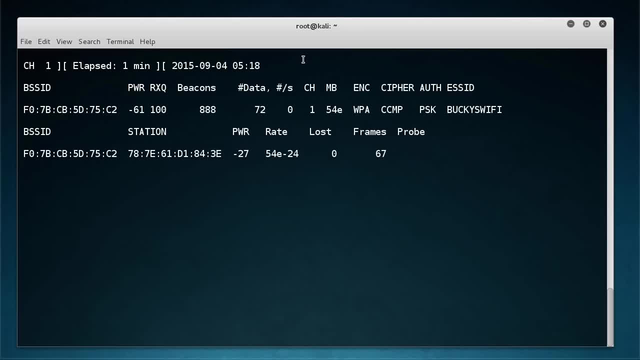 building or like a university or something. people are going to be logging into this network all the time. However, if you're a smaller establishment or maybe just like someone's home, it may take a while for someone to actually- you know- log in to the network. So if you don't want to wait, what you 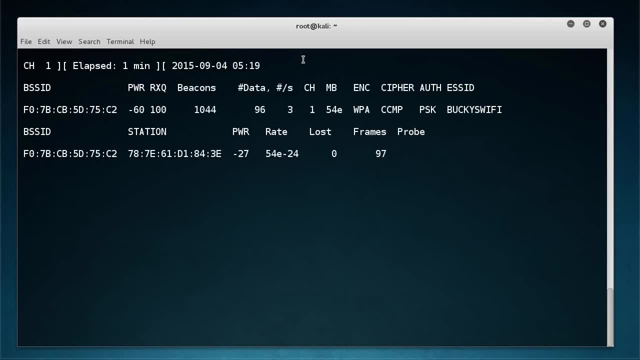 can actually do is find someone that's already connected and just send them a deauthentication packet. So then you kick them off and they're going to log back in right there. So that's a cool little trick. But take note of this: I'm picking up my tablet and I'm not connected yet. 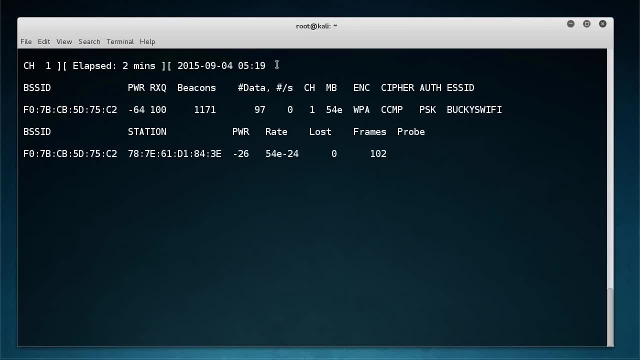 and I'm going to log back in. So I'm going to log back in and I'm going to log back in and I'm going to log back in and I'm about to type in password and log in and watch what happens in this top right. 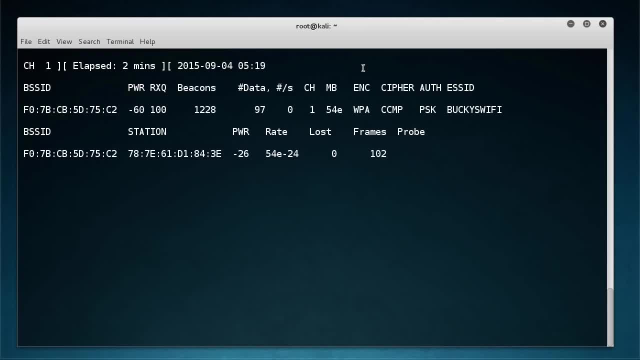 area. As soon as we capture that authentication, which is called a handshake, is going to give us a little indicator. So it's really awesome. you don't have to like: guess, did I get one yet did I get one? it's going to tell you. So I picked up my tablet and we'll just pretend like I'm a teacher. 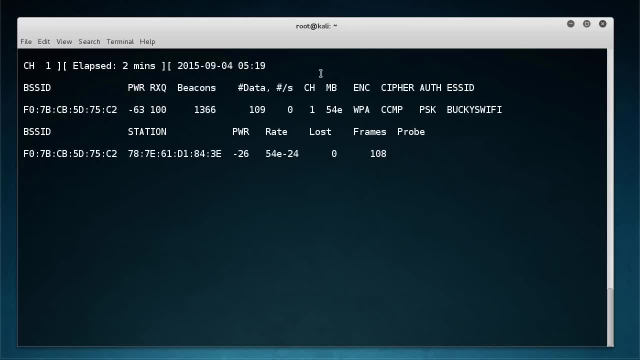 like someone legit that knows the password. Go to my settings, choose this network and then let me type in bacon. Now I'm about to hit connect and again keep your eye on that and check it out. So it says WPA handshake and this means that we did capture one. So now I can just hold down control C to stop that. 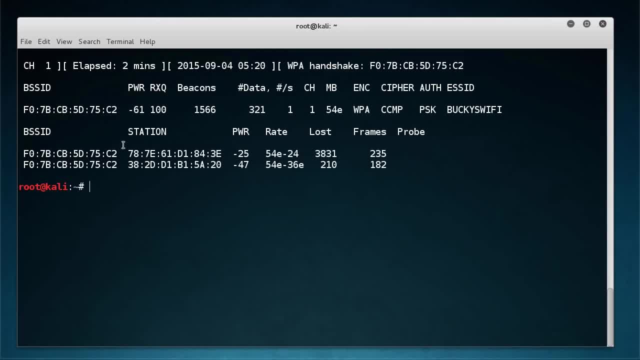 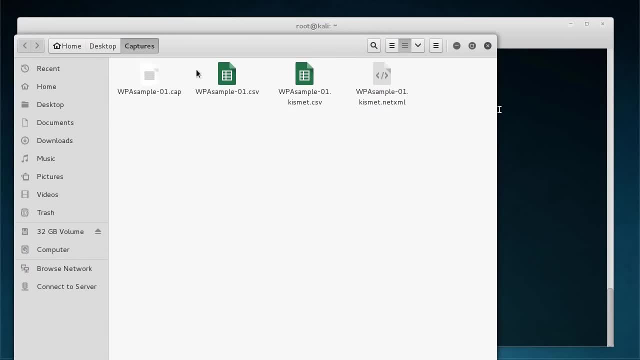 we got the information that we needed. Now, just so I can show you guys real quick, if I go to my captures right now, you see that this is the data we collected and all these different formats. I'm going to right click this and open in Wireshark. 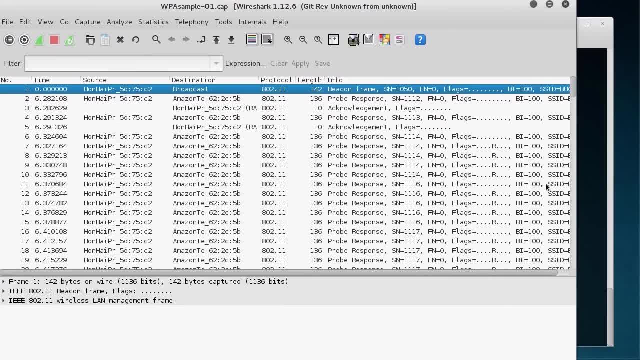 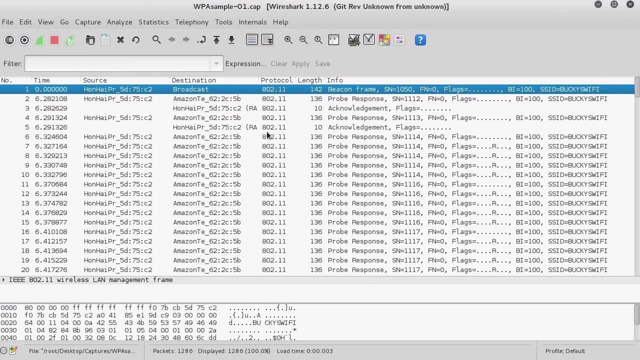 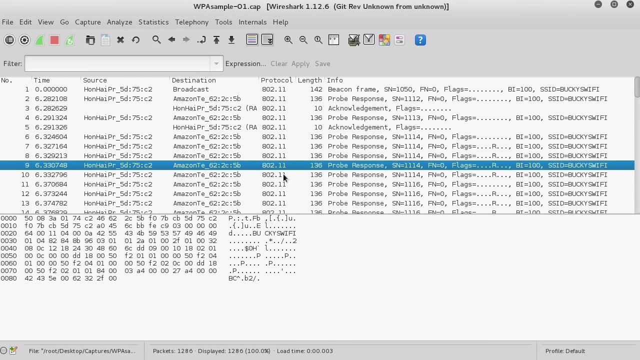 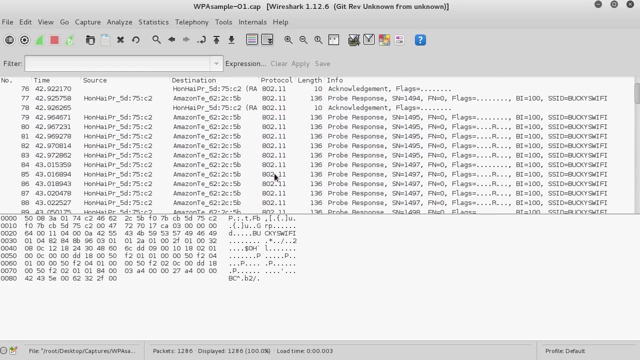 And check it out. rearrange until you guys can see. all right, So this is all the packets that we caught and if we try to read any of these, not going to be very successful. So it's pretty obvious that right now, even though we can look at, some data is, all you know, encrypted. this is useless to us, So 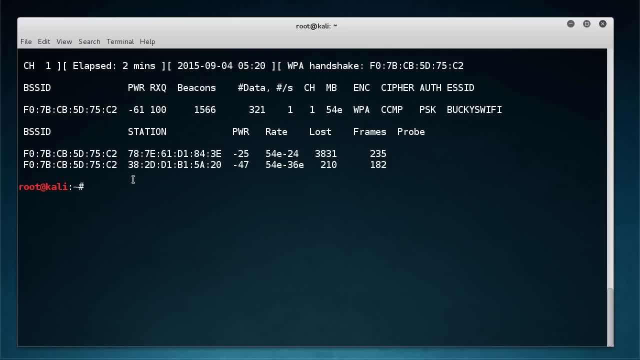 what we're about to do next is we are going to loop through the passwords And we're going to plug them each into a formula and we're going to see what one works. So what you need is actually a list of passwords, And they are all over the internet. I'm going to show you. 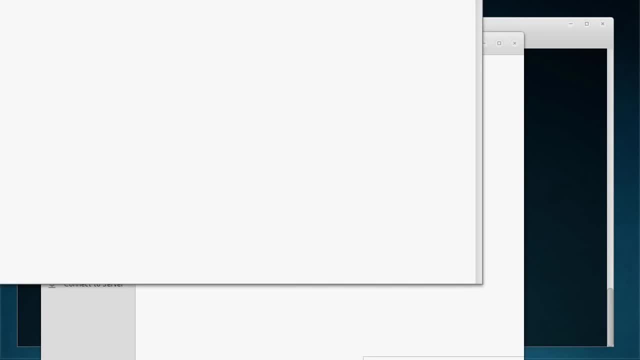 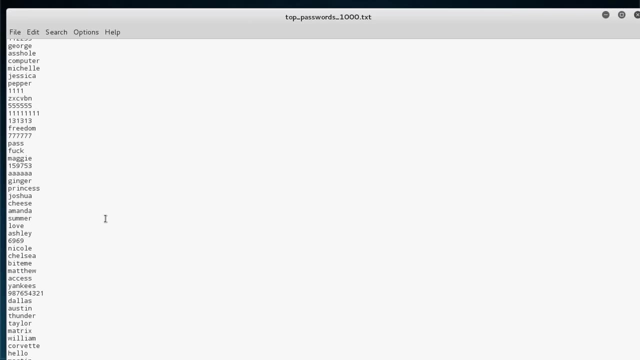 the one that I got. I actually got this off of github, So these are just the top one thousand comma ones: One, two, three. you know password one, two, three, four, yada, yada, yada, and let me Show you guys something. So I put my password online. where are you at? Where are you at? All right? 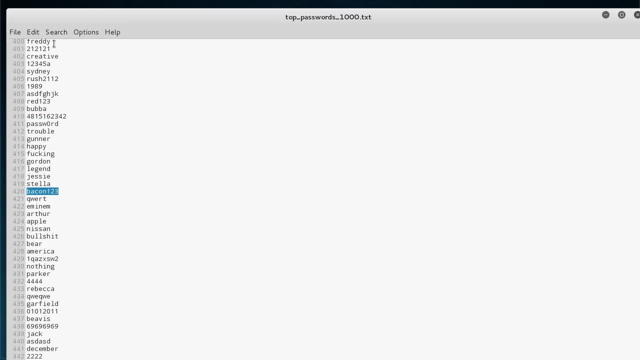 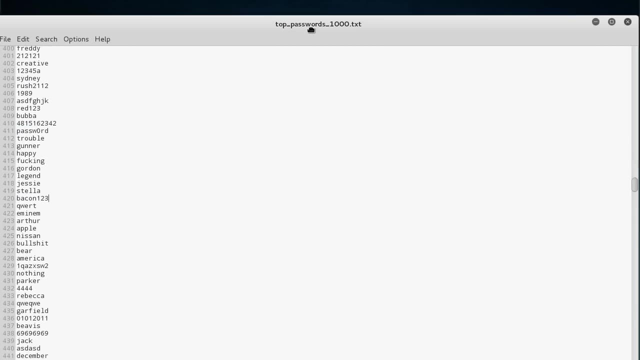 So on line 420, that's my password right here. So it's gonna try all of these and then, whenever it gets to mine, bacon 1, 2, 3. It's gonna go done Ta-da. well, it's not actually gonna make that sound, but you know it's gonna be thinking about it. 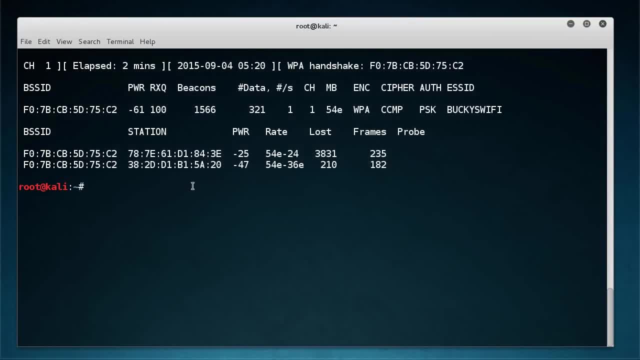 It's gonna make. hey, I found the right password, I found something that works, and This is incredibly easy. So for this we're gonna be using a tool called air crack ng. Now I'm gonna talk to you guys about a little rant. the entire suite of tools. 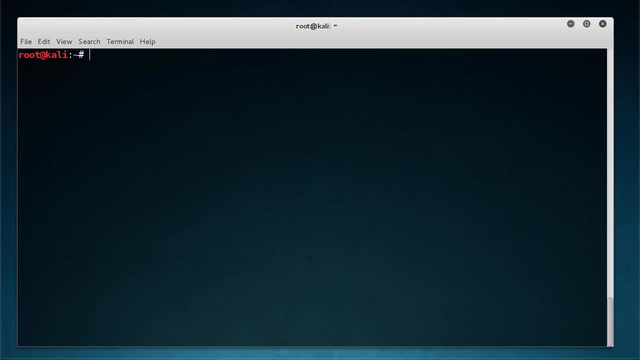 like the collection of tools that we're using for Wi-Fi. it's called air crack, and One of the tools in here is actually called air crack and G, So the name air crack isn't the name of the collection, It's also a name of a tool. 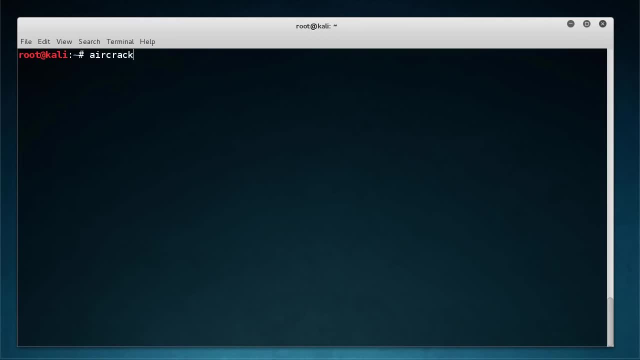 So it gets kind of confusing. but you know, don't let it throw you. so air crack ng. That's what we're gonna do- to crack the password. and then it takes two pieces of information. The first one is the capture file, the one that we just opened in a wire shop. 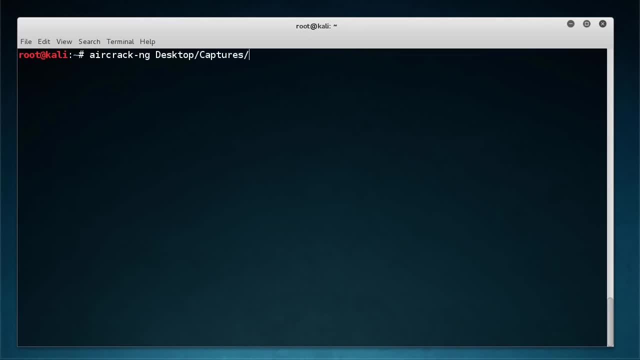 And mine is in desktop captures and it was called WP a cap. Now the next thing it needs is: alright, What are all the passwords that you want me to try? and that was that file I just showed you guys and it was desktop list and I believe was called no top. 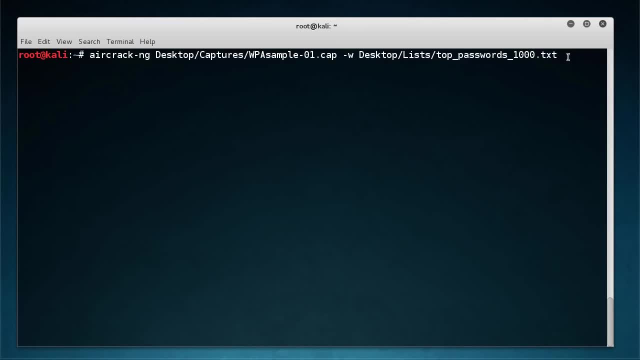 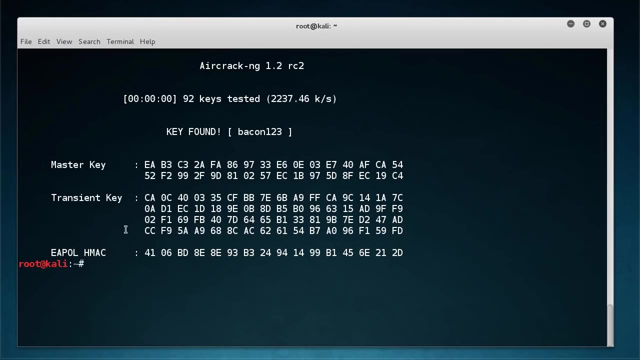 Passwords and 1000. so again, in order to find the right password, all you need is a Capture file that has the handshake in it and a list of possible passwords. I'm gonna hit enter and it's gonna start looping through those. and how quick did that take? like a second, a second and a half. 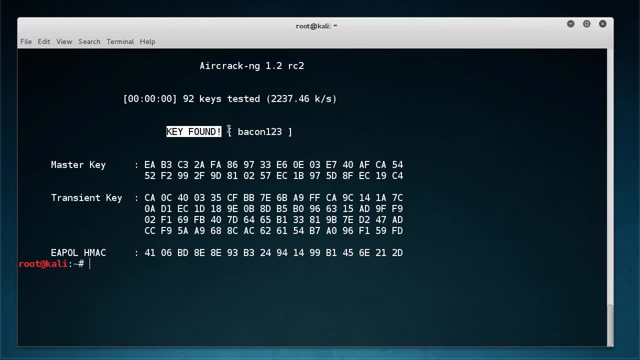 maybe, and what it says is okay. I Found your key bake in one, two, three, I mean in a blink of an eye. and, by the way, I just want to say that it doesn't usually take that quick. Sometimes people have like millions and millions of passwords. sometimes 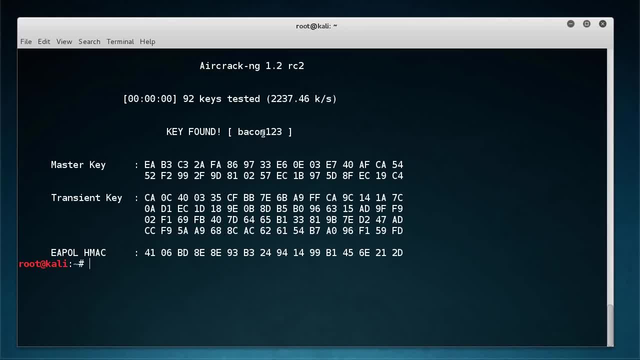 Sometimes it can take quite a long time, but I mean, this is a computer. It just ran through 400 potential options in like half a second. And I mean, if you ever looked at anyone's password on their Wi-Fi, they're usually not that complex. 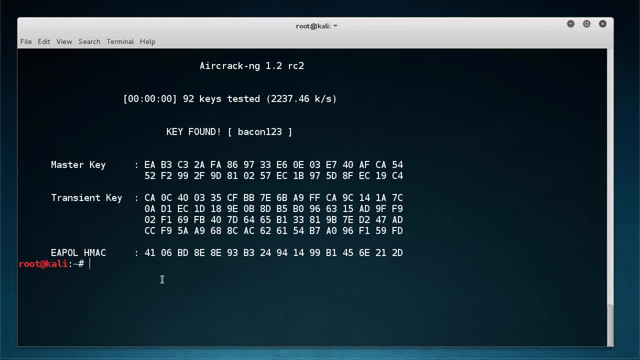 like the majority of people. So that is how you perform that. Now, what I'm gonna do, now that we have the password, is: we now have all the pieces that we need. Not only can we log in to the network just using this password, but we can also start decrypting. 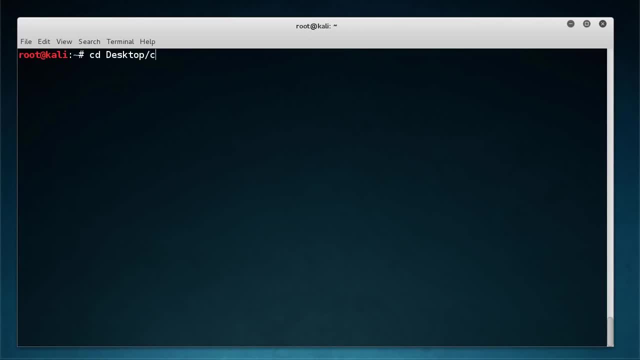 all of that information. So now let me move over to my captures file, And what we can do here is we can run a tool called airdecapng, and this is a tool that you use to actually decrypt those packets. So now that we have all the pieces, 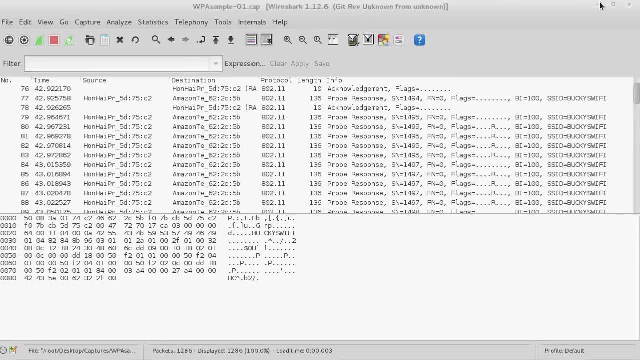 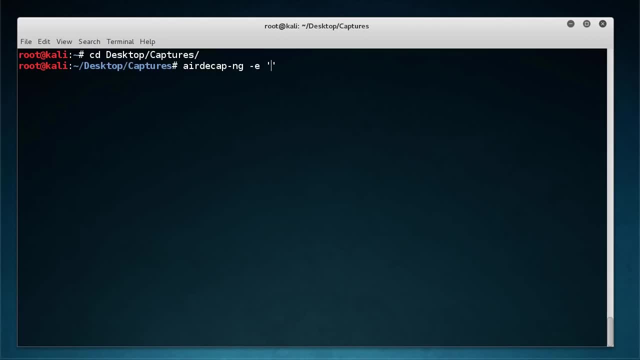 what we can do is we can start looking through these packets and decrypting them. Pretty awesome. So the formula takes a couple pieces and we already have all of them. The first thing is what's the name of the network? So it was Bucky's Wi-Fi, simple enough. 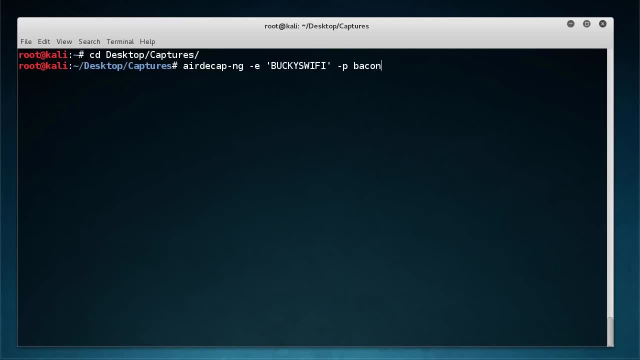 Now, if you write minus P, another piece that it needs is the password for that network, And we just figured that out. it was bacon123.. And the last thing you need to give, of course, is a file that you want it to decrypt. 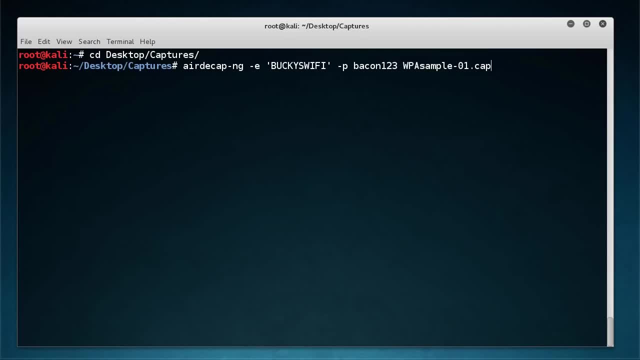 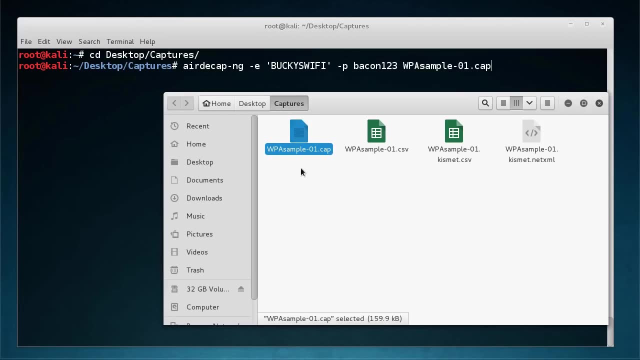 So mine was wpasamplecap and check this out. So keep an eye on this, because what it's gonna do is it's actually gonna build a whole new file, but this is gonna be with decrypted, So the file names are kinda similar. 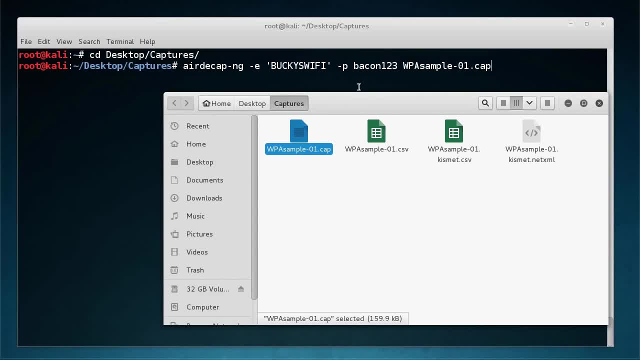 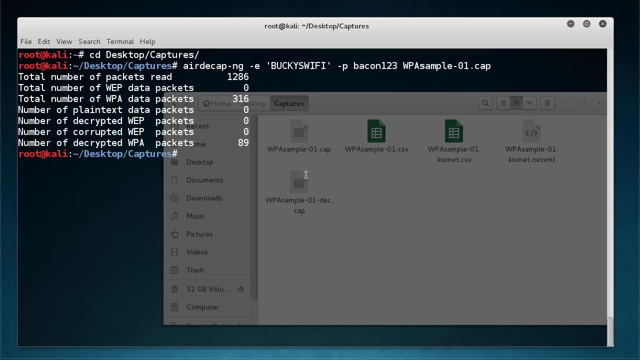 It's gonna name it the same thing as this, but put a minus DEC at the end. So keep your eye on this. whenever I run this command, Gonna hit enter and you see that it generated a new file. Well, if I let me just open that up in Wireshark.